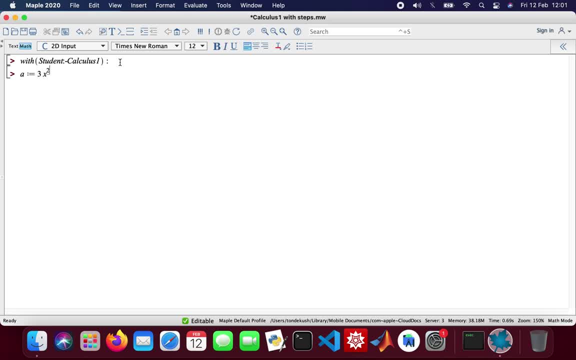 some random number. 3x squared minus 2x was love X, then B, the schools, x times sorry times, 2x, okay, and then F be sine 2x and then my G, that'll be 2x cubed, okay, plus 4x squared random number 9. so I'm gonna make this more. 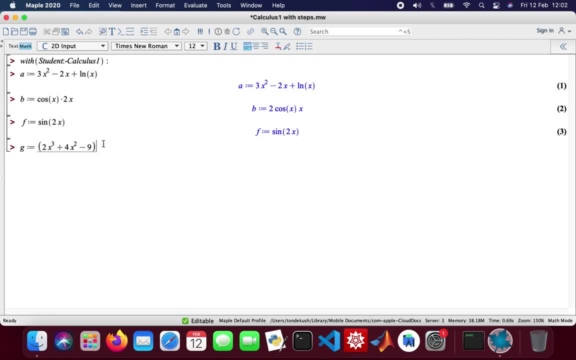 interesting. then divide that by x squared minus 4. okay, right, so I'm gonna sort of differentiate in some of the functions. so what I'll do is uh, type in a div and then now a with respect to X. this is what I get, and then, if I don't do the differential tutor so div, so you can see. 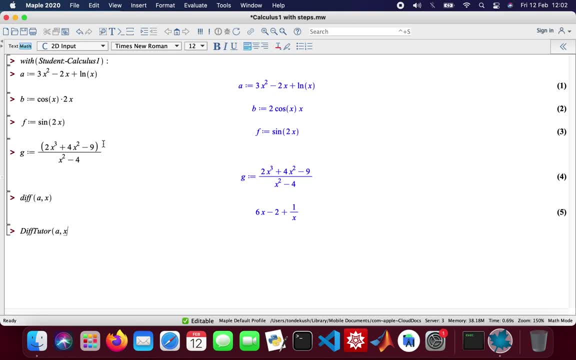 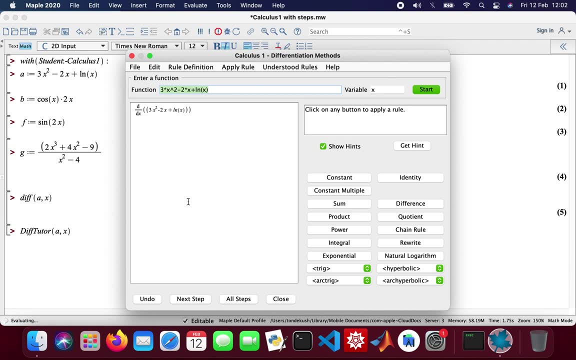 the steps a with respect to X. so the pop-up comes up and then it tells you what goes on. so you just click on next step, keep clicking it and this rectangle box will show you what's going on, and then keep doing that. then here we are. so 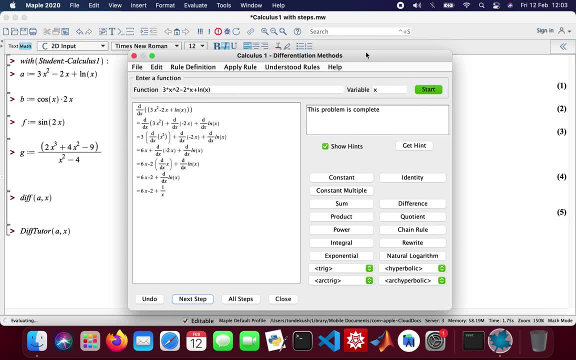 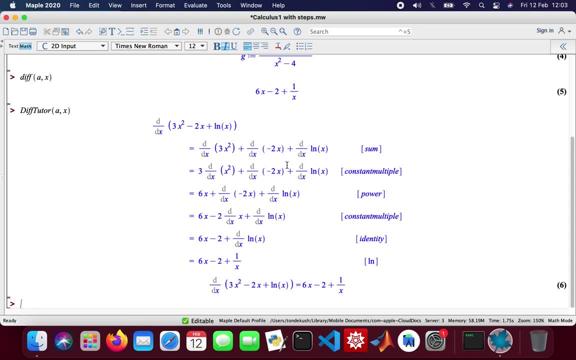 that's the final part. so that's all answer there, and so here we are, okay. so if you click on close, it imports that into into the worksheet, okay, so I'll do my B function again. so so that would be B. I'm sorry, diff, and then B with respect to X. okay, and then diff to that. that's B with. 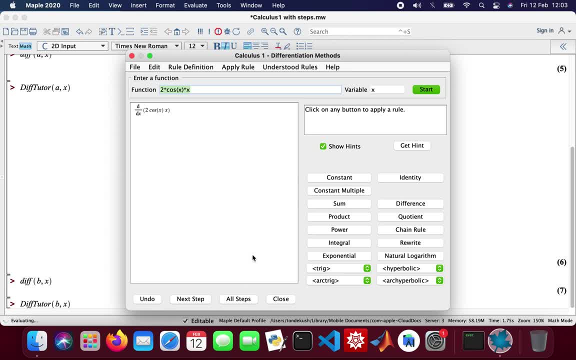 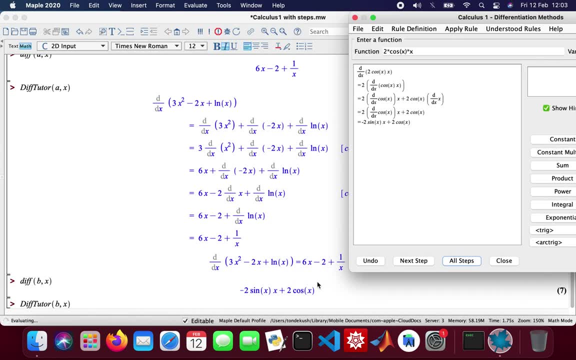 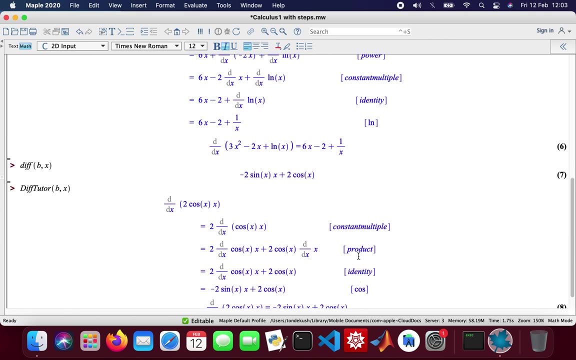 respect to X. so it's pretty much the same thing that I did earlier on. so so here we are, okay, then click on close and yeah, so it tells you all the steps of what's going on. okay, right, so, um, I'll do my g1, because that's not onto the f1 as well as well. 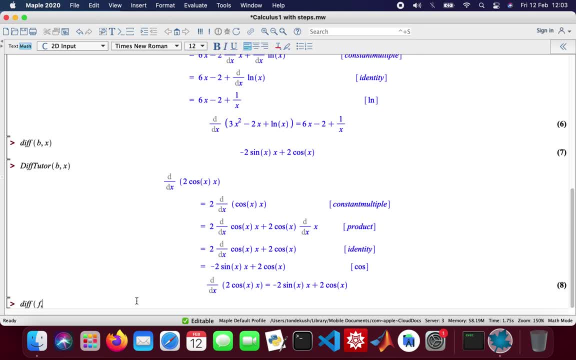 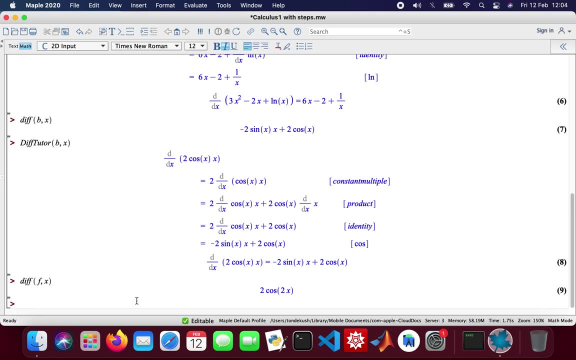 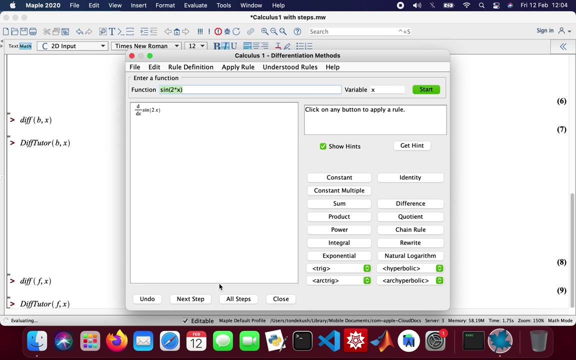 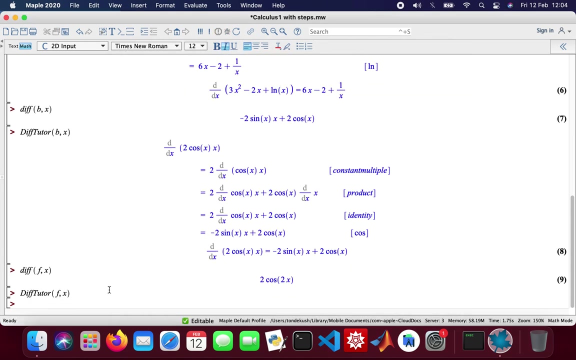 if okay, and then do the differential tutor right. so all the steps. so here we are. so, essentially, if you just, if you just close it like that, if you just do that, it doesn't import anything. so you know. so if you want to import something, just click on the close button, okay, and then. 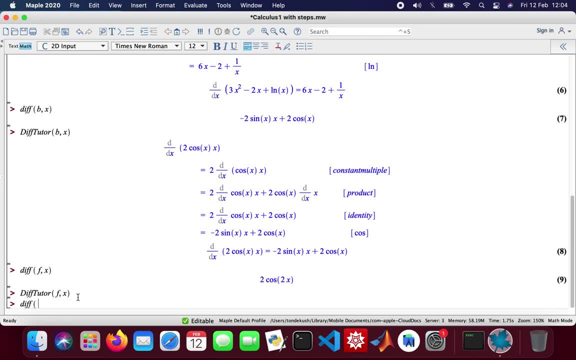 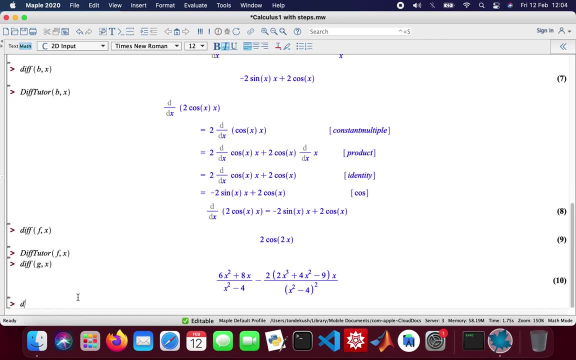 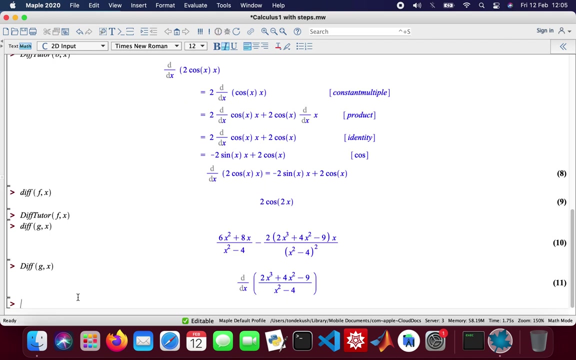 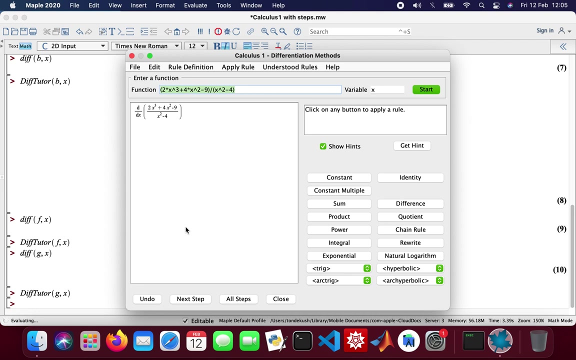 my G sort of, then G with respect to X, okay, and then I'll do the differential two does well, you, sorry, you caught my bad, sorry, yeah, yeah, yeah, it got there, okay so. so these are all the steps, okay. so, if you did this the first time, done in g b's. 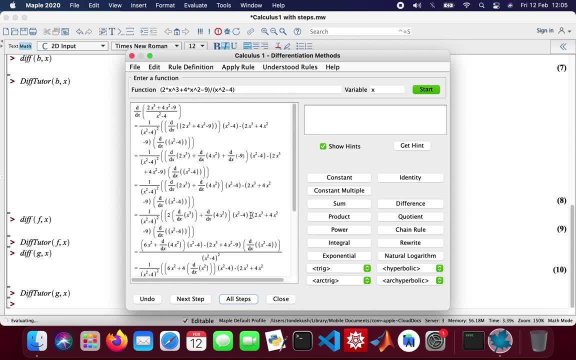 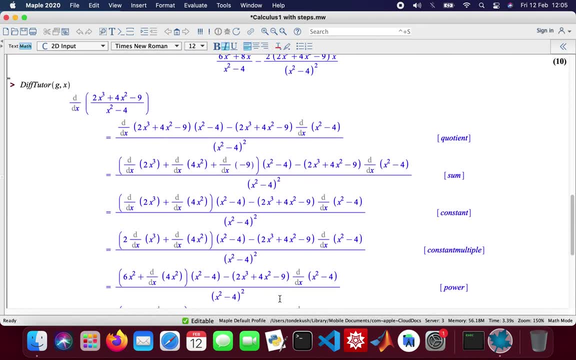 perspective, then if you were to trace it back to that edit, you wouldn't be a very good. so, like I said, if you click on that it doesn't import anything, but if you click on that, you will import everything into your worksheet. so so these are all the 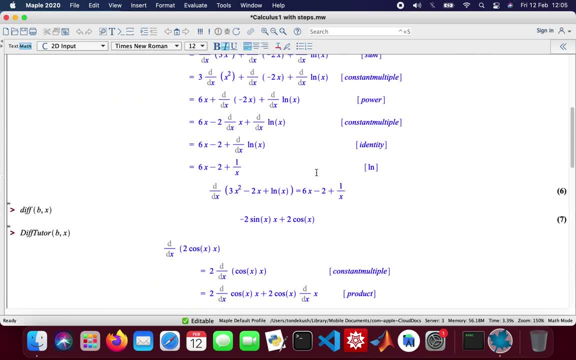 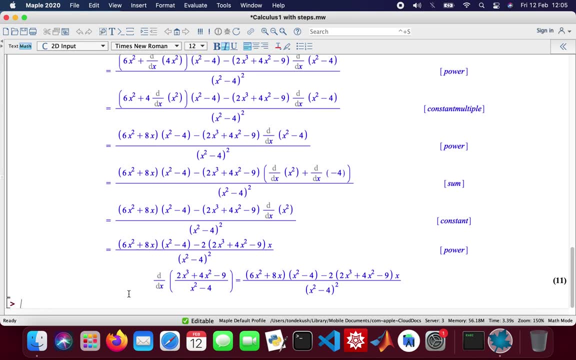 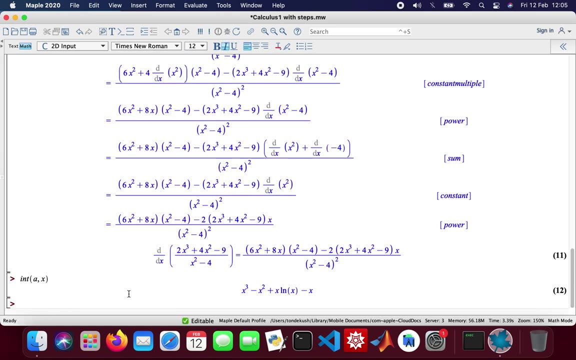 steps until you get your final result. so this is using the caution rule anyway. okay, so now I'm going to do the integrals. so I'm just going to integrate the same functions, so int, then a with respect to X, and then I'll do the two. 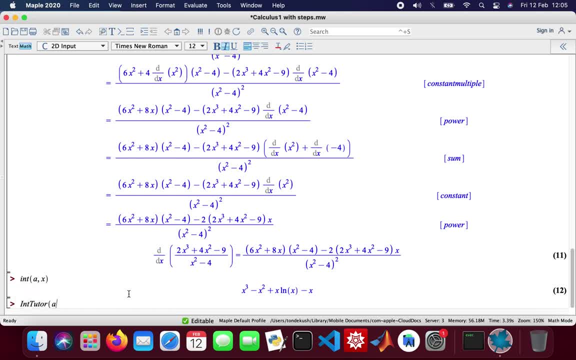 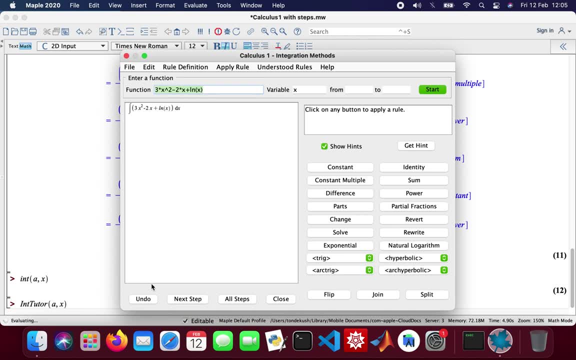 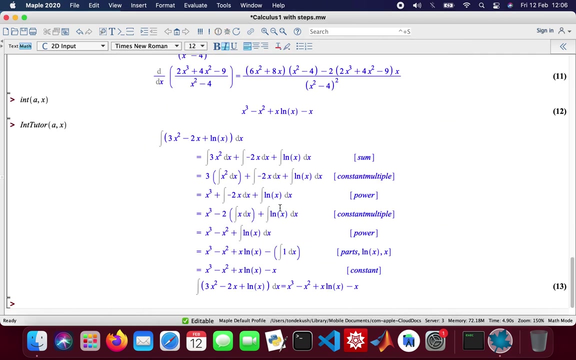 as well. a with respect to X. so that's the indefinite integral. okay, so it's the next step. so you keep doing that if you want to see the steps. okay, so here we are, so I'll close that. then it imports that into your worksheet so you can see. 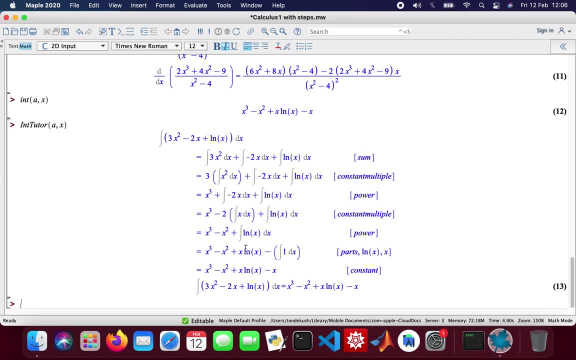 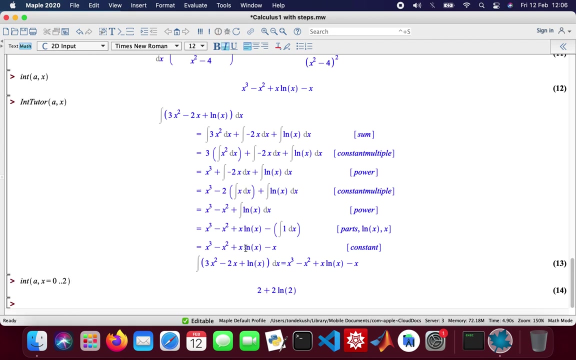 what's going on, okay, and then probably going to try and to let me do the one limit. so okay, so I'll do so. int then a, so X equal to zero, to two. okay, then I'll do the two as well. you, you, what I'm going to do is go to the next step and I'm going to do the two as well. 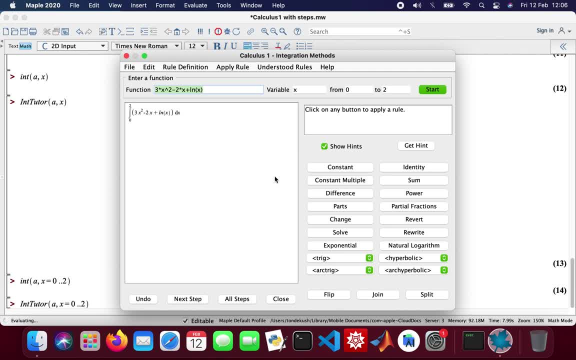 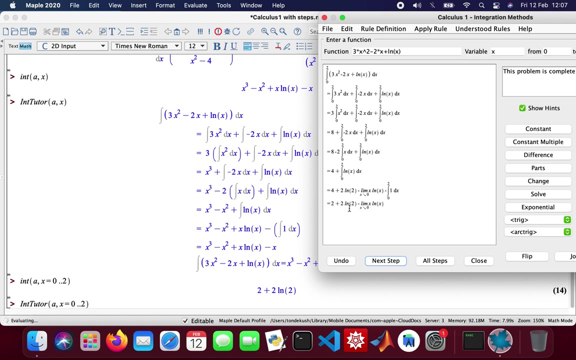 so there's, that's a variable X from zero to two. so that's a definite integral, okay. and then next step: it's essentially the same, but then off. so for applying your limits, right. so that's it. the problem is complete, okay. so obviously that that's zero. so you get that two per second, okay. so that's the next step. and 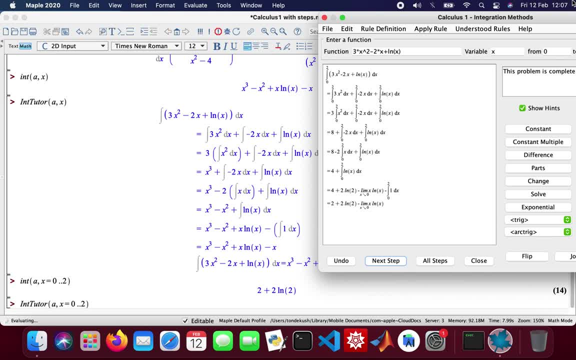 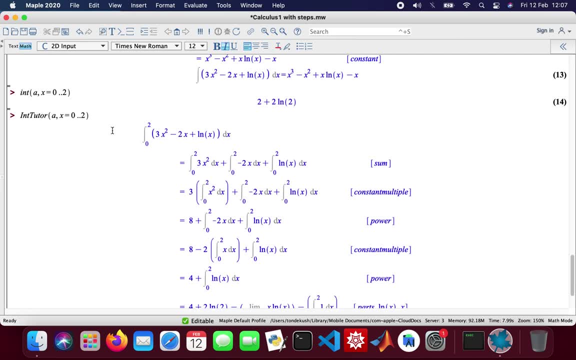 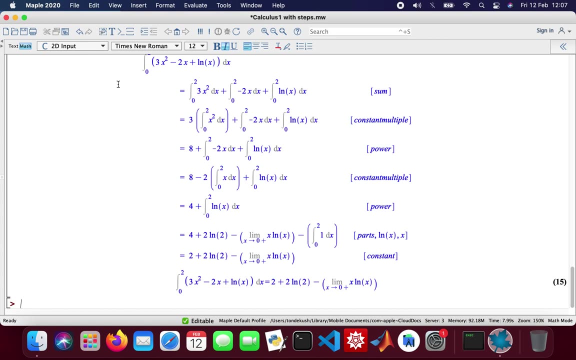 then next step is essentially the same, but then off. so if I apply it to a limit 2 times log 2, okay, and I'll close that. then it reports that, so it shows you all your steps of how you solve the problem, okay, and then I will do my f function as. 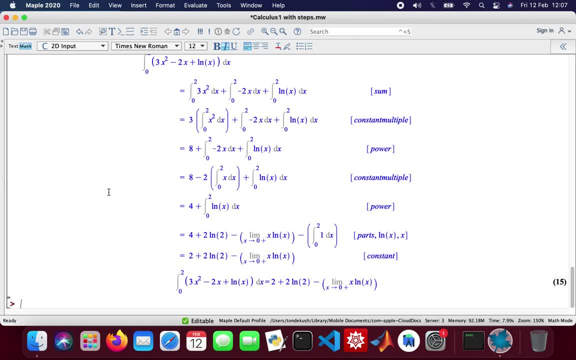 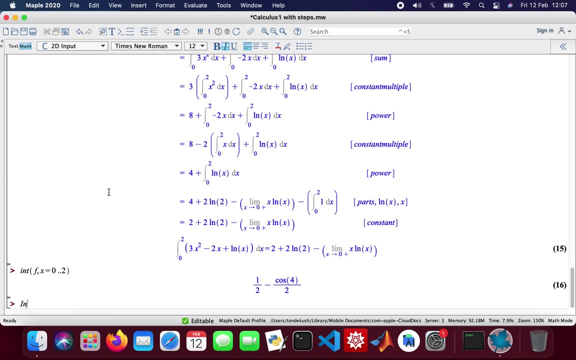 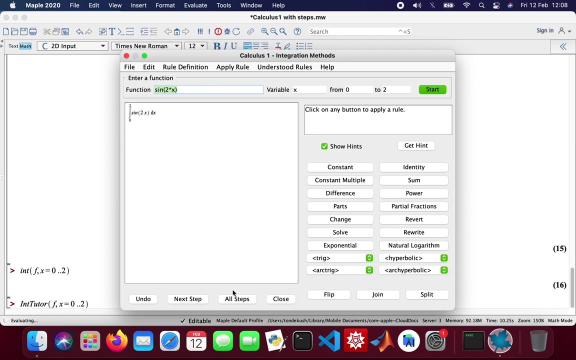 well, just to show you, like you know, just to find out. so, and I'll use limits this time. so X equal to 0 to 2, okay, and then the Tudor part, my X values take, you know, 0 to 2, so all the steps. so here we are.